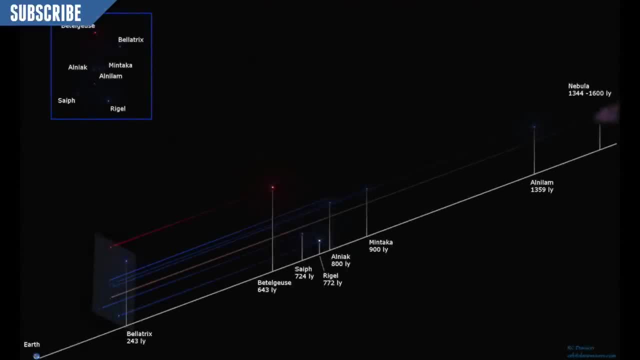 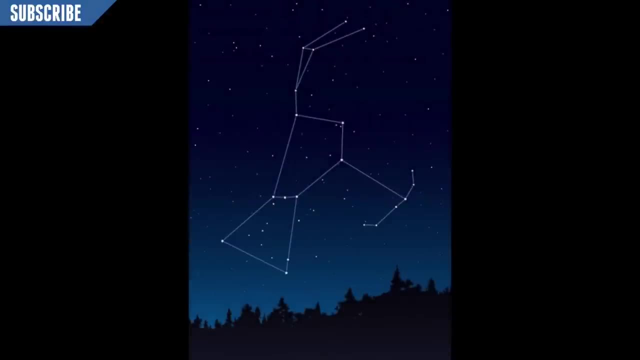 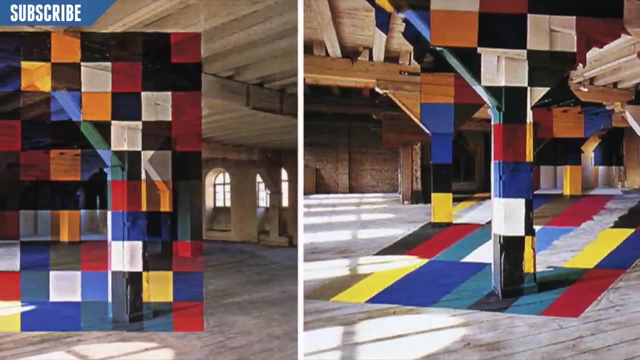 it from a three-dimensional point of view. we can see that some of the stars are nowhere near each other But, seen from Earth, are a perspective. they line up perfectly to show the constellation. It's very similar to a perspective piece of art. From one angle it can look completely random, but 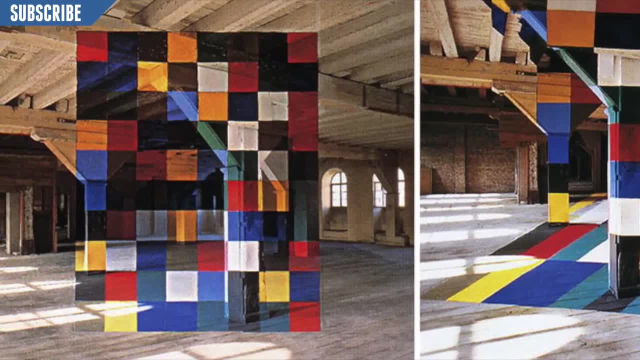 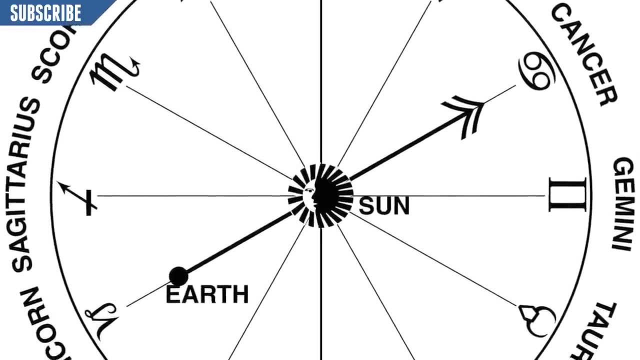 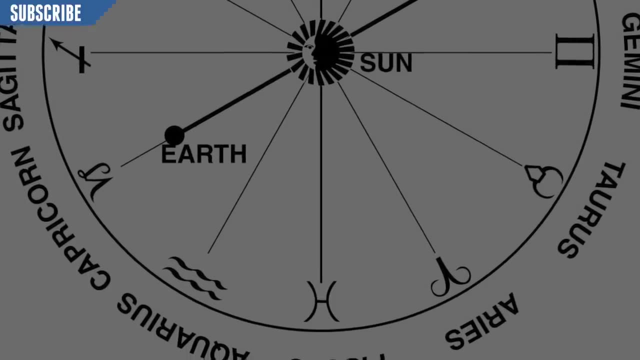 from the right perspective, everything lines up and the picture is created. Since the earth is moving around the Sun, we see all of the constellations in the sky. at various points In the past, people actually use this information to tell the seasons from one another. Many of these people actually use constellations. 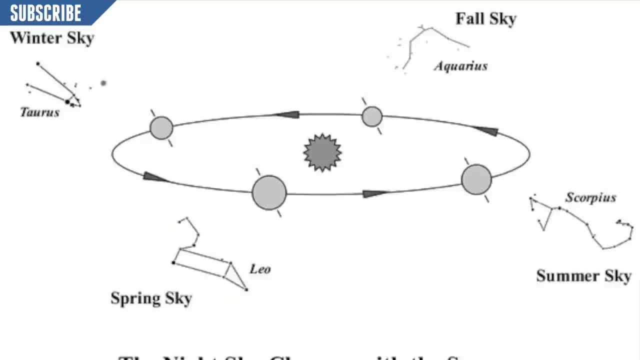 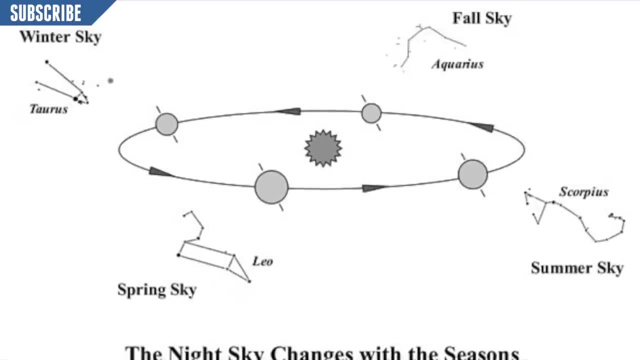 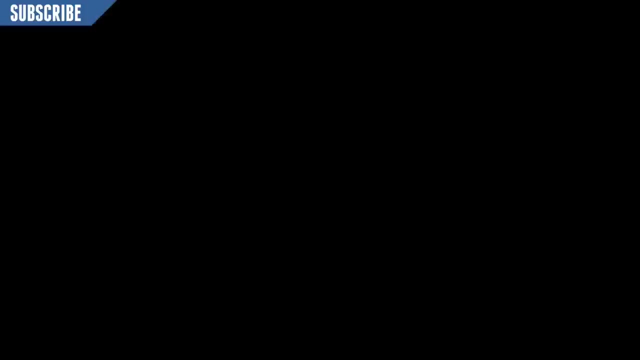 to actually map and build structures to understand these constellations, and this was to observe and understand the movement of the constellations. In some cases, these maps were actually built to alert them when there was a change in the seasons, For example, when winter turned into spring, Almost every advanced. 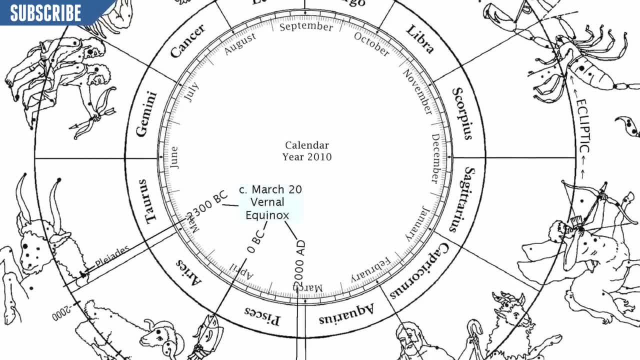 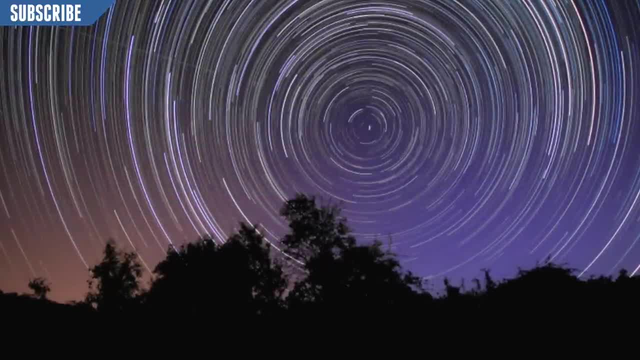 culture around the world used constellations and also navigating the oceans. Constellations were actually used to help ships from one location to another. The crew members on the ship knew how to read constellations so that they could change course based on the pattern of the stars. 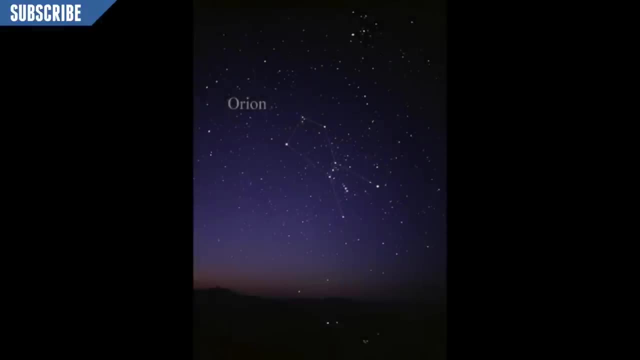 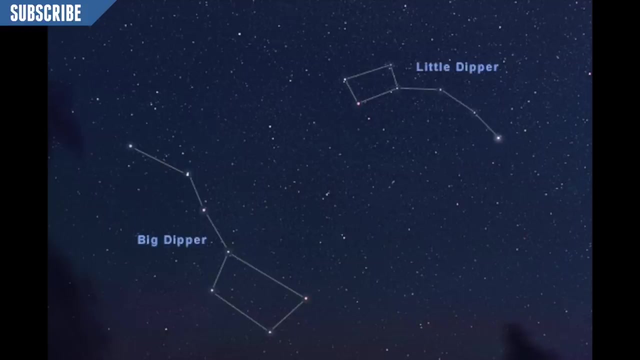 and where they were in the sky. There are a lot of famous constellations, For example, Orion, Leo, Gemini, the Big Dipper and the Little Dipper, But because we all live in various parts of the planet, we actually see constellations in different. 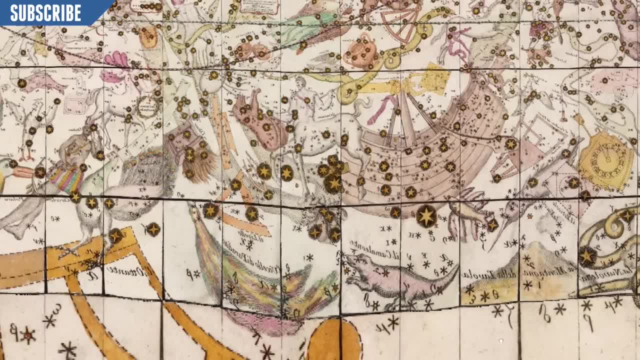 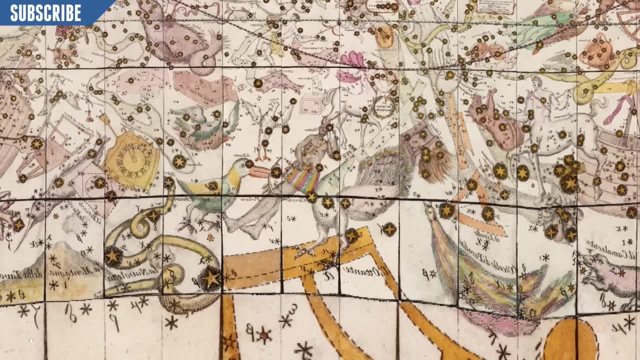 places in the sky. The names for these constellations have actually stayed from the past. This is simply because it's a bit of a tradition, and they've already been established as these names, Even though some of them don't really look like what they're. 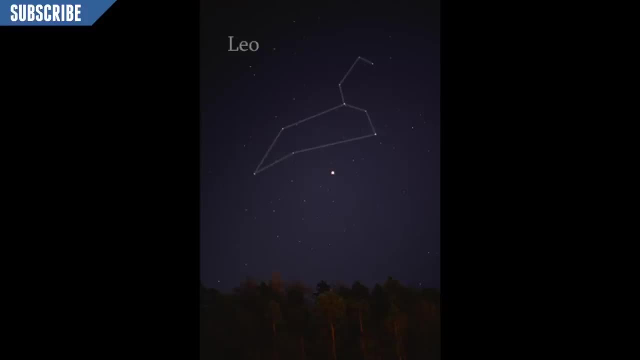 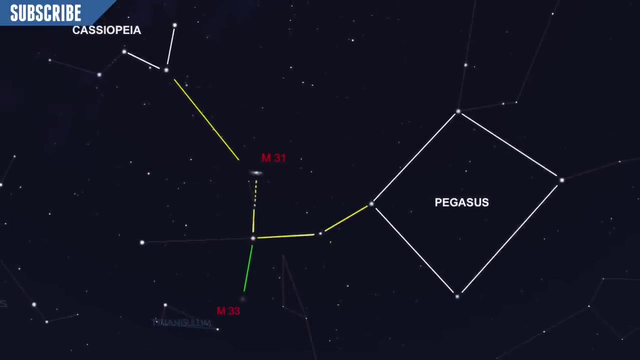 trying to describe. I mean, that doesn't look like a lion to me, But in modern astronomy it's just a great way to navigate around the night sky And for a beginner in astronomy it's just a really good way to get used to how the night 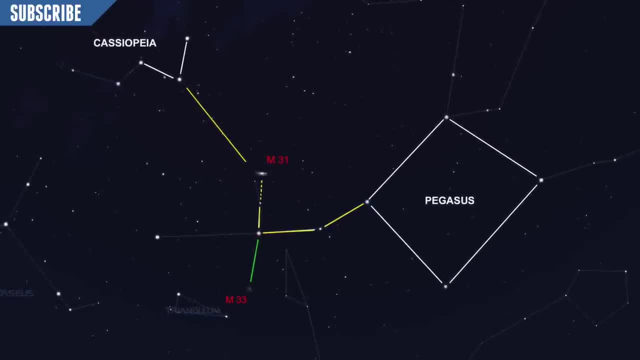 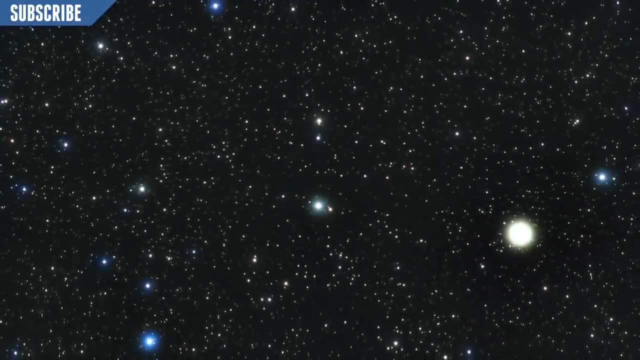 sky looks, Even though most of it is just simply dots and lines. So I hope that's given you a great understanding into what constellations are and also these mythical creatures from the past, Or, as I call them, just simply dots and lines that